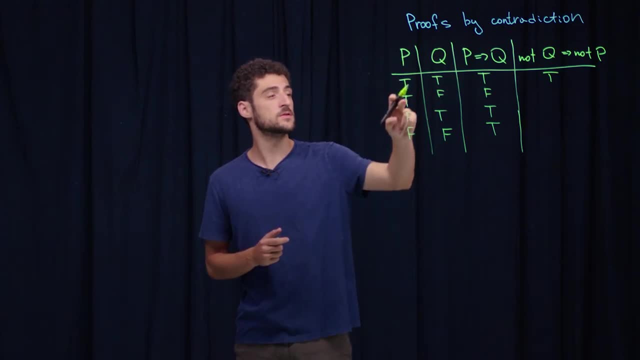 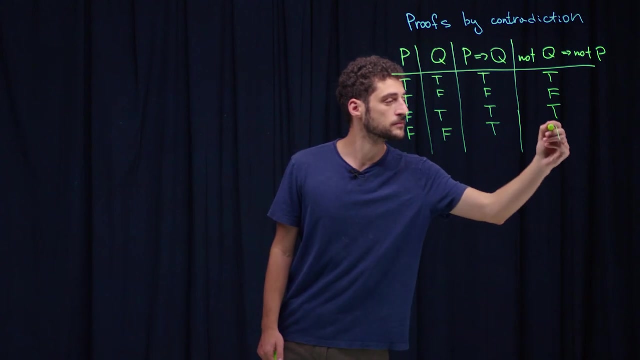 If q is false and p is true, then it's in the form. true implies false, which is false. In the case when q is true, we know that not q is false again, so it's true. If q is false and p is false, both of them, when they are negated, are true, so it's true. Now we may. 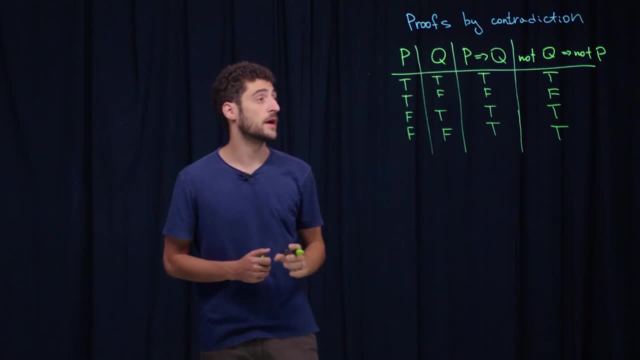 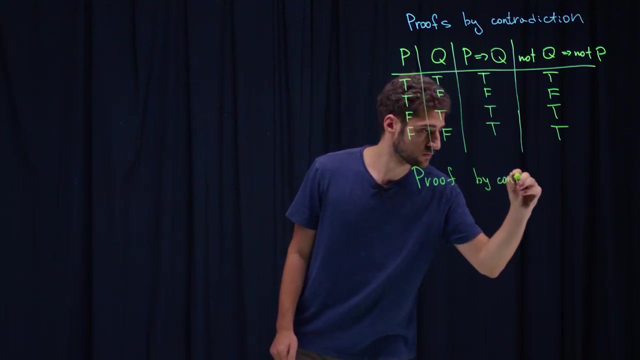 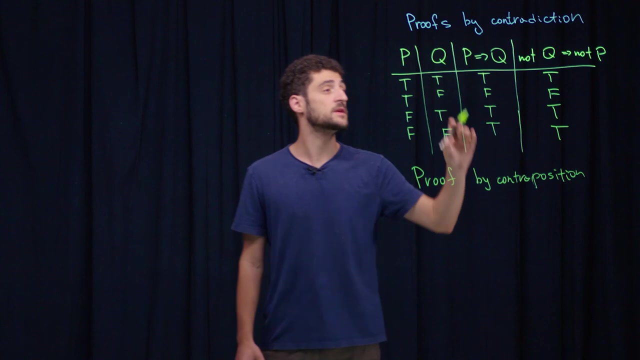 notice that these two columns are the same And if you want to prove p implies q, it's the same as proving that not q implies not p, And the method that facilitates this is called proof by contraposition. It's called like this because not q implies not p is a contraposition of p implies q. Okay, let's. 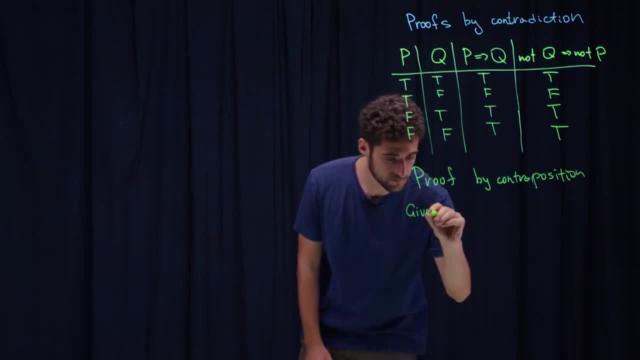 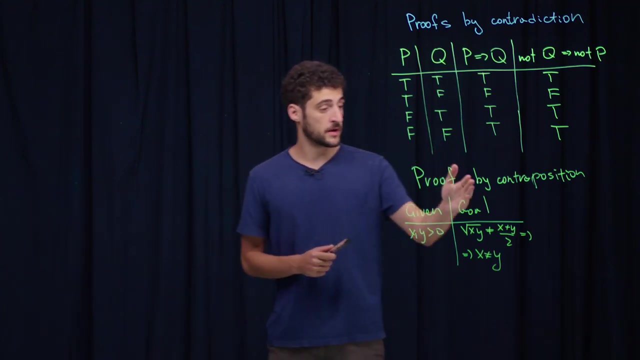 give an example of this method. So it's given that x and y are positive reals And the goal is to prove that if square root of x, y is not equal to x plus y over 2, then x is not equal to y. Okay, So, since we are going to prove it by contraposition, 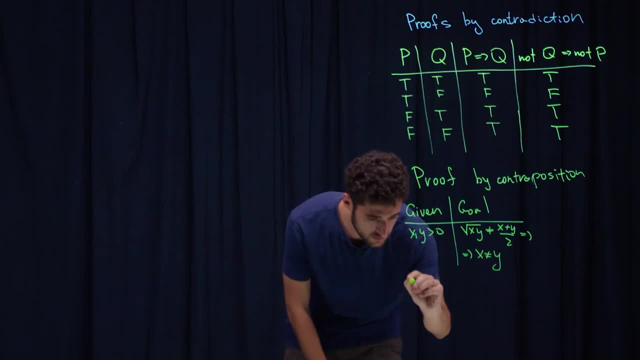 it means that we need to write p and q and see what are them. So p, here is x plus y over 2, is not equal to x plus y over 2.. varwick feeling to square root of x, y and q here is: x is not equal to y. S calculated on number ofけれ宗. 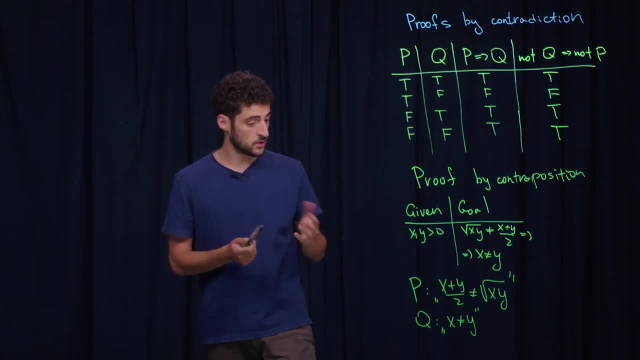 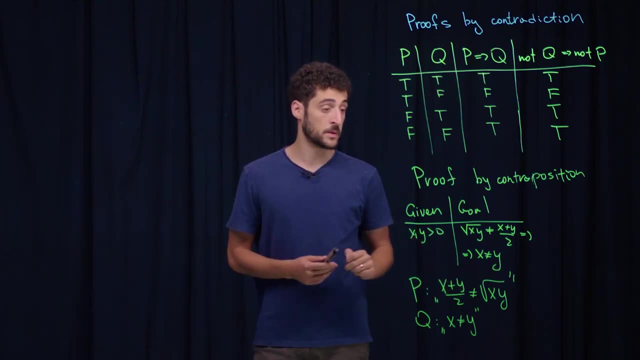 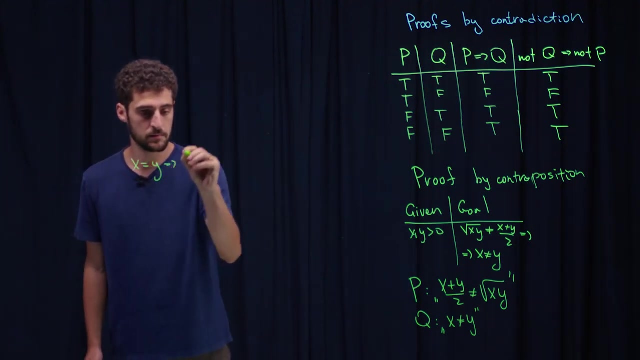 while Note that not q implies, not p- is the statement that if x is equal to y, then x plus y over 2 is equal to square root of x- y. Let's try to prove this. So we know that x is equal to y and it implies that, first of all, that's an liar- that x is. 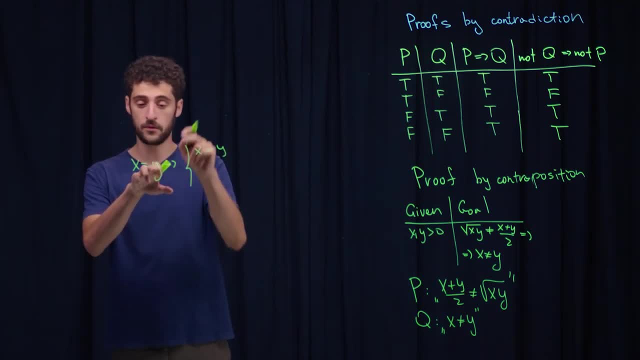 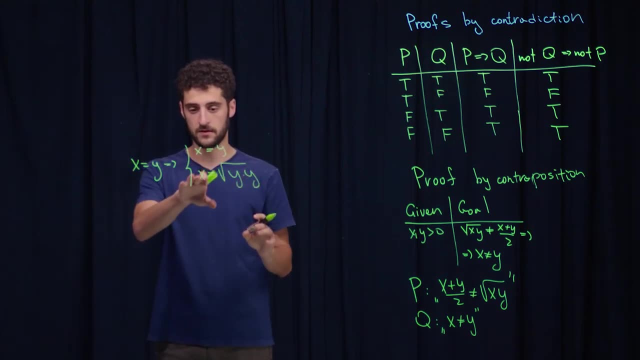 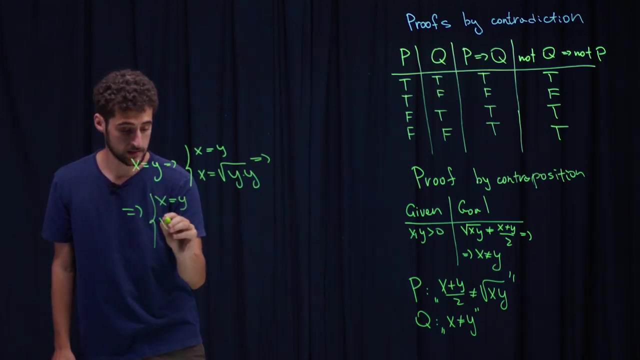 equal to y, and also we may replace y, square root of y times, y. Okay, Now let's modify the left side So we get that x is equal to y and x plus x over 2, which is equal to x, is equal to square root of y times. 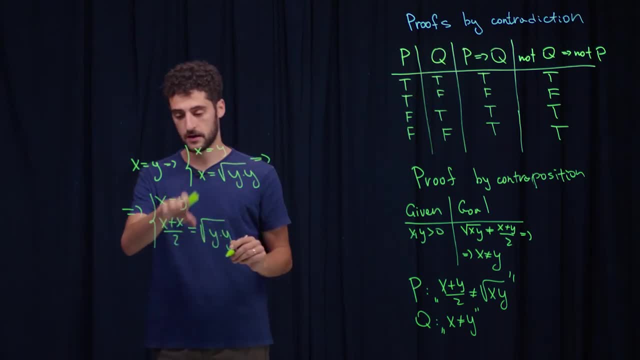 y. Now we want to replace this y by x and this x by y and get this Okay. So we prove that x is equal to y implies that x plus y over 2 is equal to square root of x- y, And it's the same as not. q implies not p, And it means that we prove that p implies q And 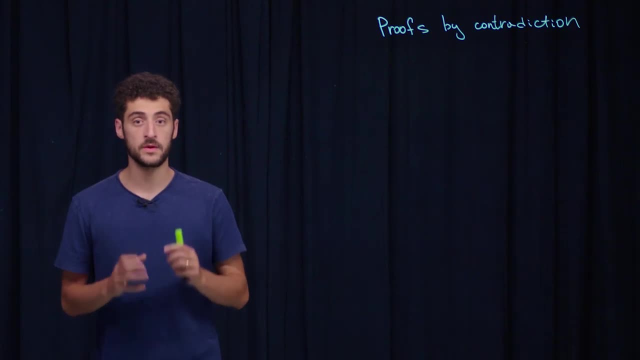 it's the same as not q implies not p And it means that we prove that p implies q And it finishes the proof. Unfortunately, not always we want to prove that P implies Q or something in this form. Sometimes we want to prove some statement like just P. 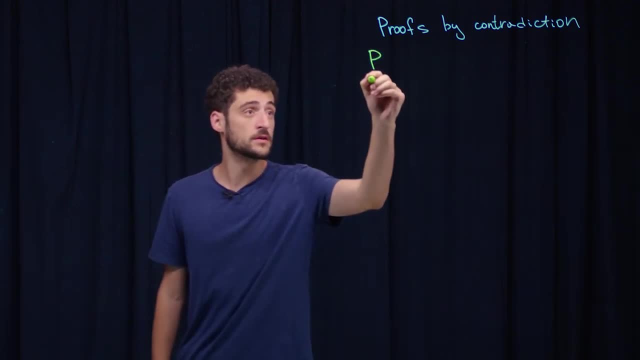 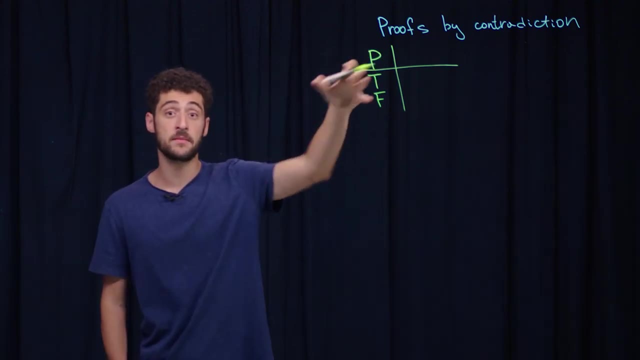 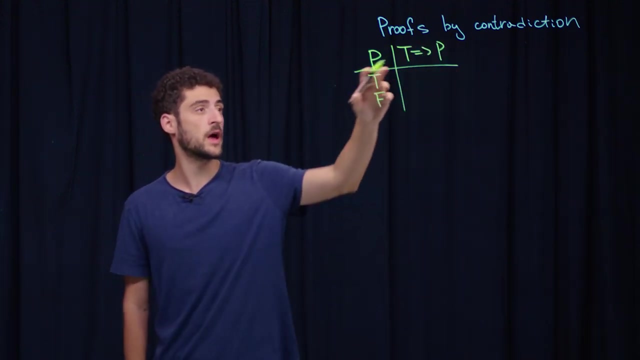 So what should we do in this case? Okay, note that truth values of P may be true or false and we need to somehow replace P by an implication. Note that true implies P is an implication and truth values of these statements are the same. 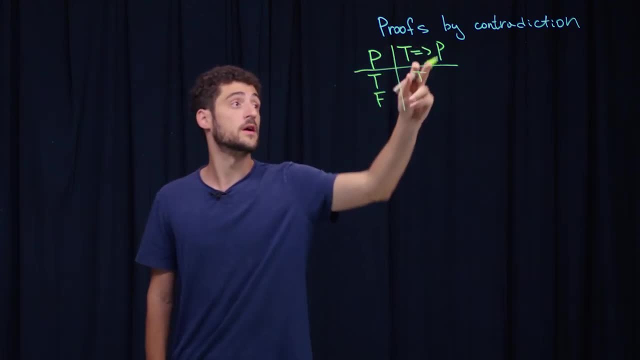 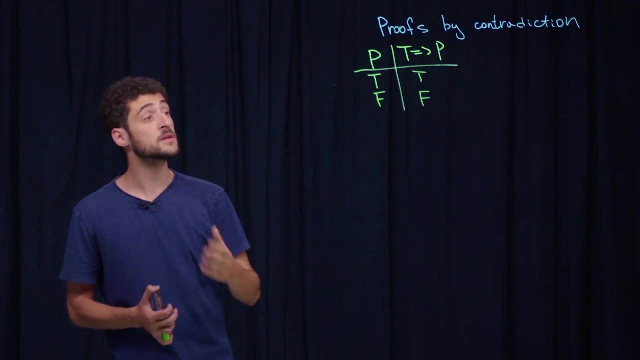 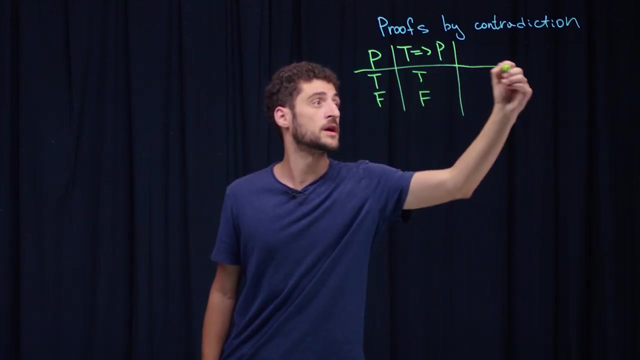 because if P is true, then true implies true is true. If P is false, then true implies false is false. Okay, so now we write our statement in the form of implication and we can use the proof by contraposition And note that it's the. 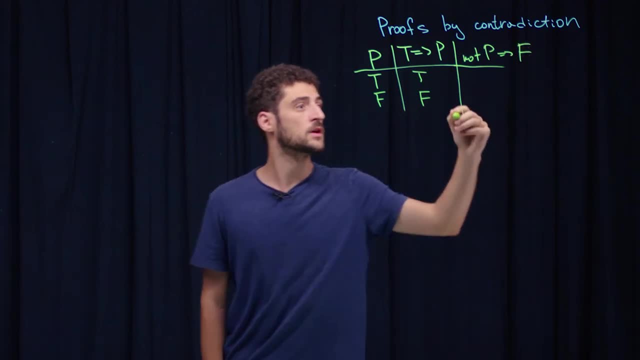 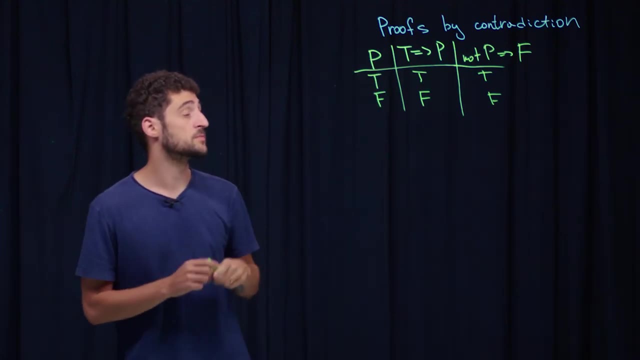 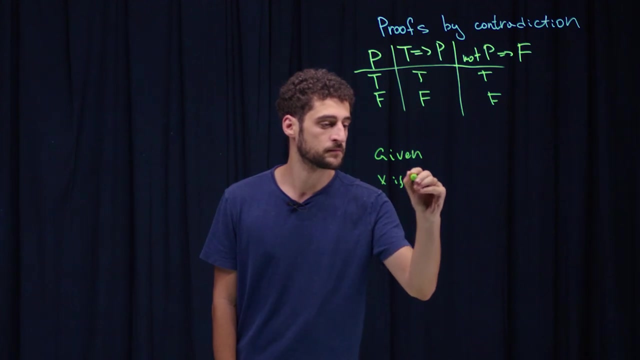 same as not. P implies false, which is true and false respectively, And this method is called proof by contradiction, because false is a contradiction, It's a contradictory statement. Okay, let's give an example of how can we use this. So let's assume that we are given that X is real and the goal 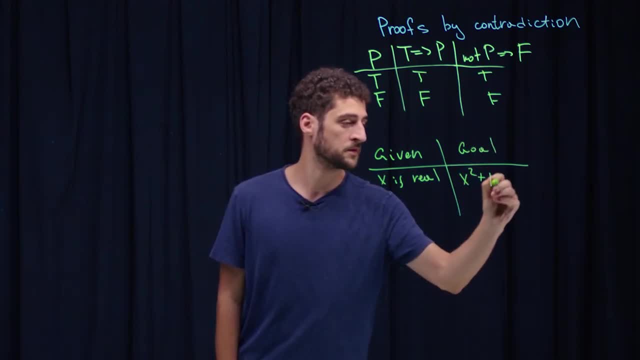 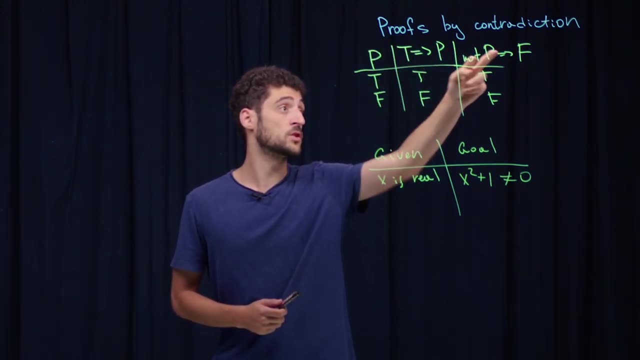 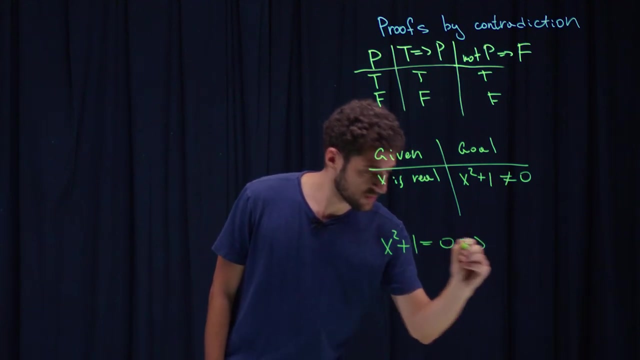 is to prove that X squared plus one cannot be equal to zero. Okay, guess what? we're going to use a method We possibly never survive. OK, Since we are going to use this method, we need to start from. not P or X squared plus one is equal to zero. 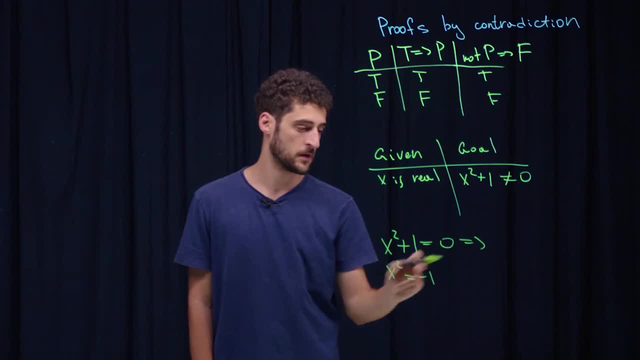 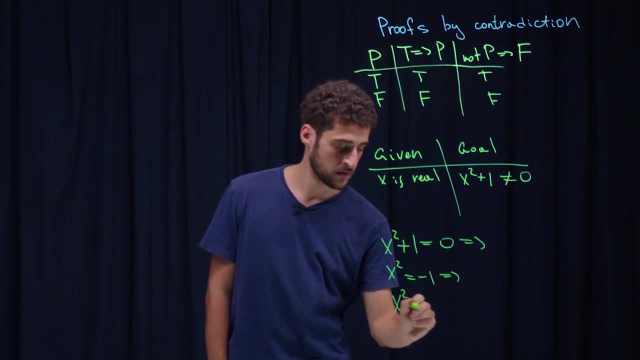 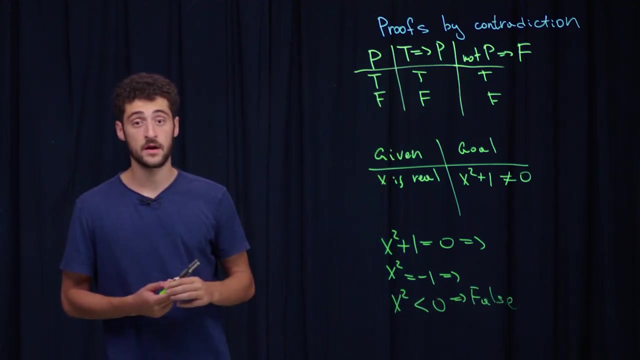 It imply that X squared is equal to minus one, because we can use this one and write it on the right, And since minus one is negative, it's the same as X squared is less than zero, which is false. Hence we know that squared real number is always non-negative.